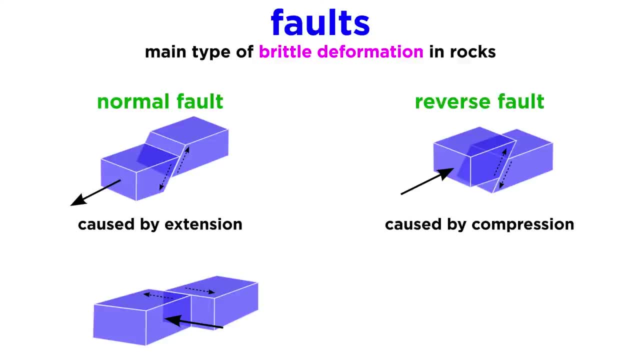 by extension, reverse faults by compression and strike-slip or transverse faults by shearing. Normal and reverse faults are called dip-slip faults because fault motion or slip is parallel to the fault's dip. This is in contrast with strike-slip faults where slip is perpendicular. 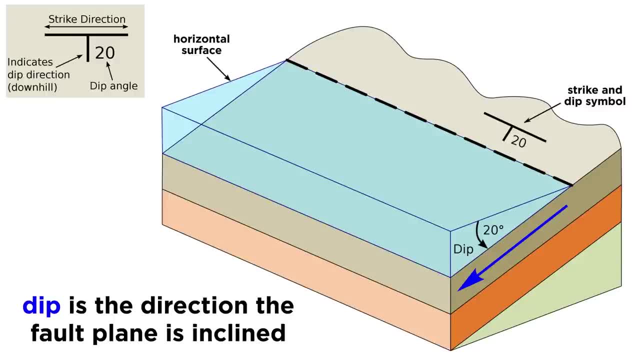 to the dip. In geology, dip refers to the direction that the fault plane is inclined. To conceptualize this, imagine that you pour a cup of water onto an inclined surface. The direction that the water flows is the dip, which has two components: an azimuth representing 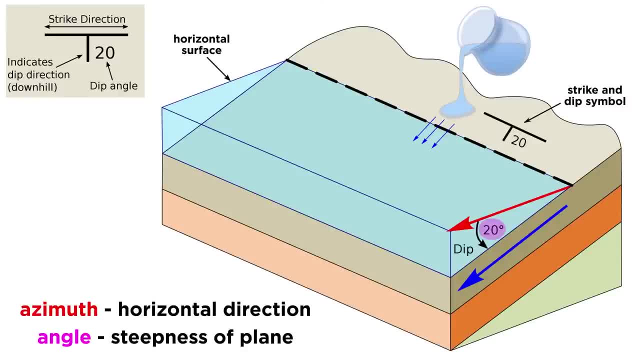 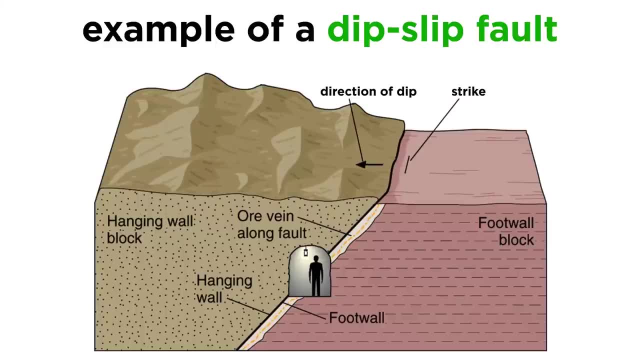 a horizontal direction and an angle representing the steepness of the plane. In any dip-slip fault there is a hanging wall and a foot-wall. If you imagine drilling a tunnel longitudinally through the fault, when standing in this tunnel you would be standing. 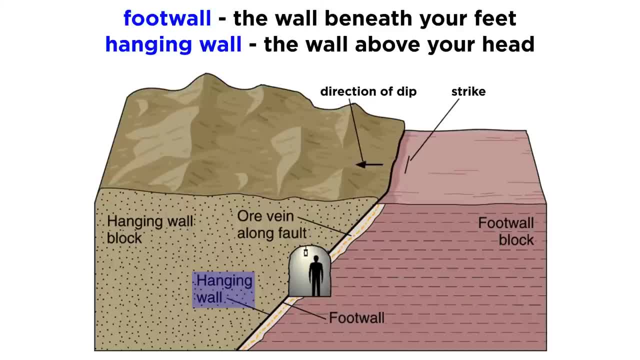 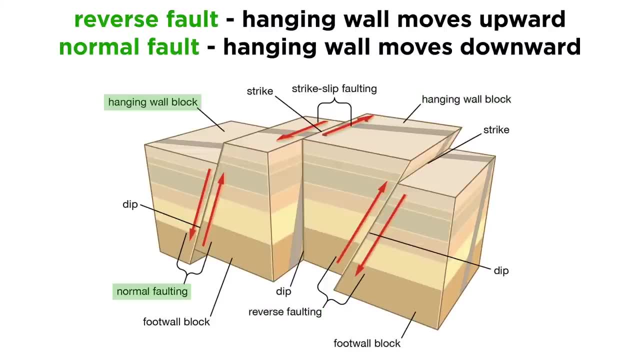 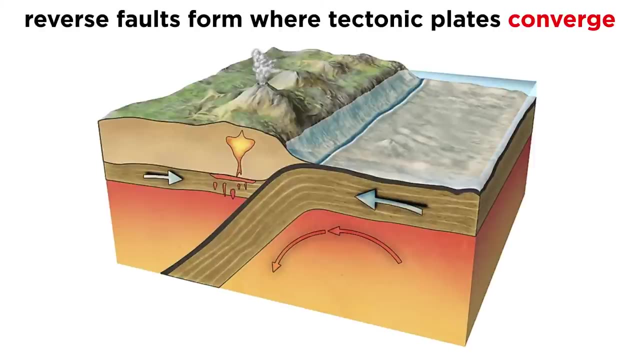 on the foot wall and the hanging wall would be above you. In reverse faults the hanging wall moves upward and in normal faults it moves downward. Reverse faults primarily form in areas where the tectonic plates are converging, like along subduction zones and continent-continent. 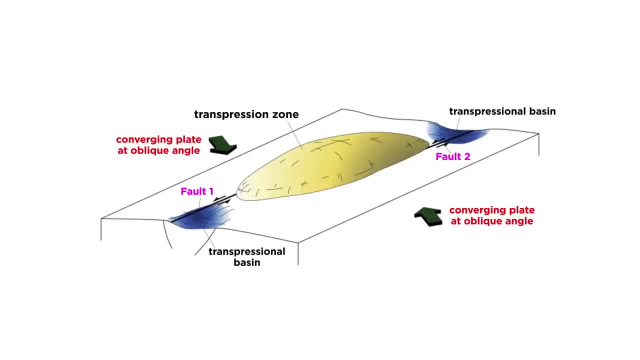 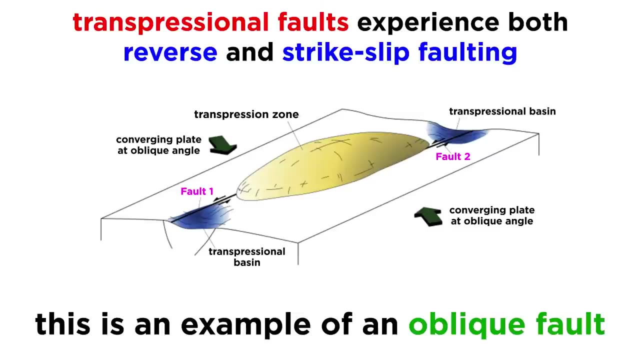 collisions. There are also areas where the plates are converging at an angle. These transpressional faults experience both reverse and strike-slip faulting. A fault with both dip-slip and strike-slip motion is called an oblique fault. An example of this is the San Andreas Fault Here, the Pacific. 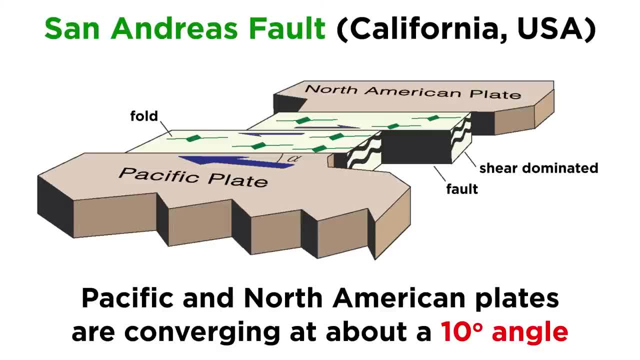 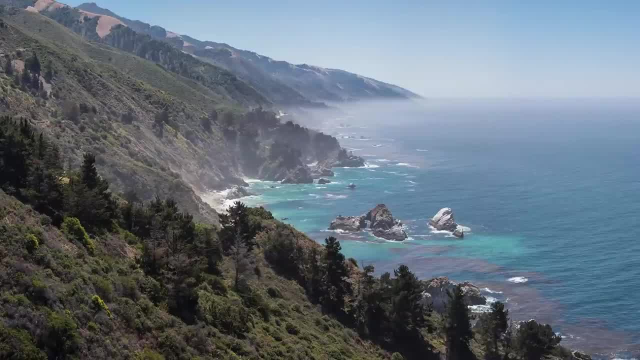 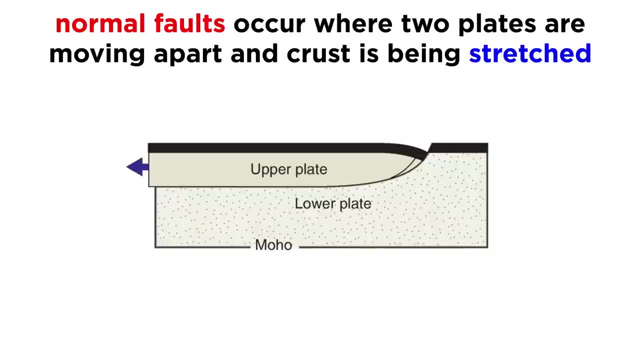 and North American plates are converging at about a ten degree angle. Though predominantly a strike slip fault, it is also slightly compressional, as is evidenced by the coastal mountain ranges of California. Normal faults are most common where the plates are moving apart and the crust is being stretched. 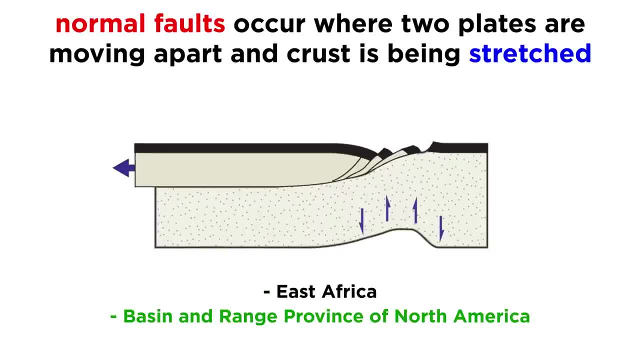 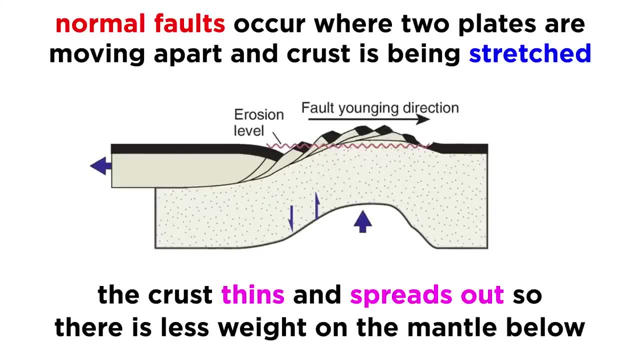 This is currently occurring in East Africa, the basin and range province of North America, and at the center of every ocean basin in the world. As the crust thins during extension, its weight above the underlying mantle is reduced and spread out over a larger surface area. 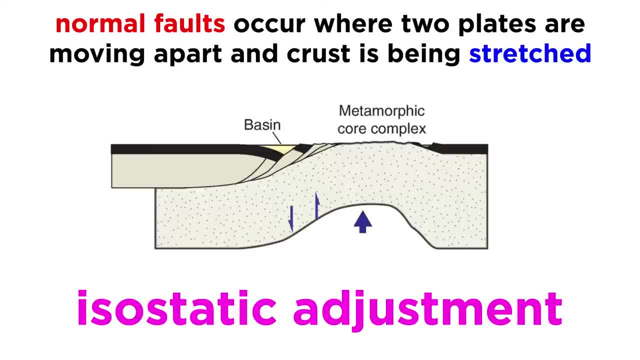 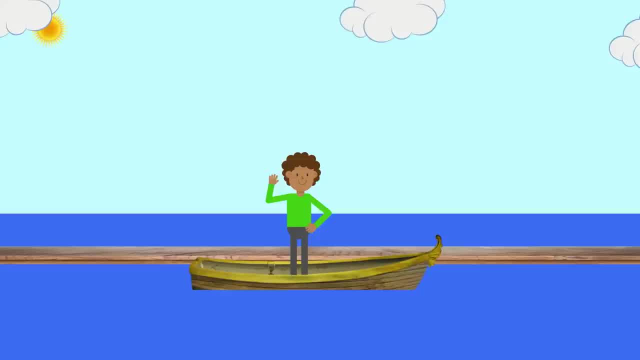 This causes the crust to bob up in a process called isostatic adjuvation Or, more specifically, isostatic rebound. It's like walking off a boat: When your weight is removed, the boat bobs upward and rises in the water. Get back in and the boat bobs down in response to your weight. Back to the geological 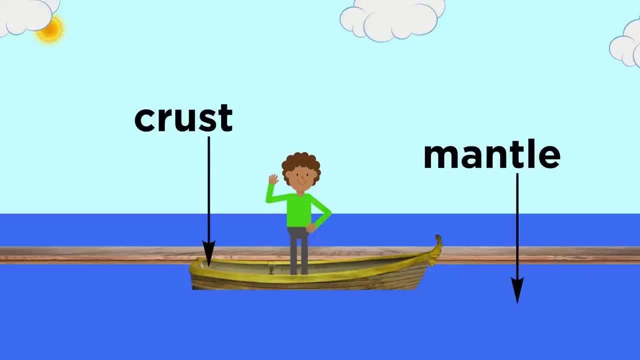 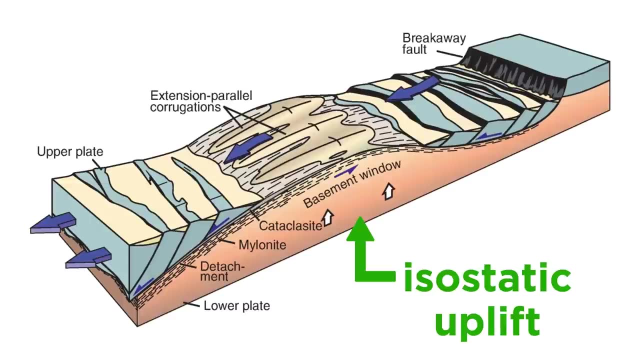 case, the crust is analogous to the boat and the mantle is analogous to the water, with the crust bobbing up and down in response to the thickening and thinning of the crust. The same thing occurs in areas that are experiencing compression: The compressional. 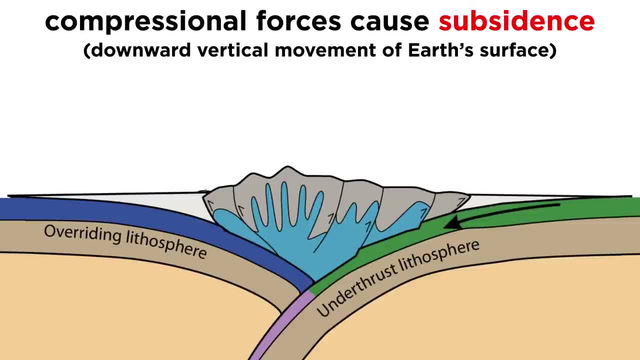 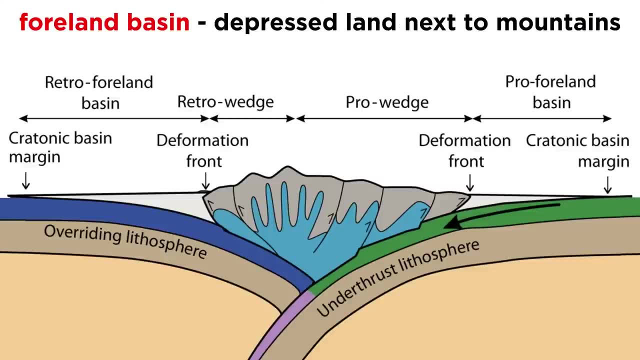 forces thicken and shorten the crust, causing subsidence, because the now heavier crust will sink in to the mantle. This is what leads to the development of foreland basins or large areas of depressed land located adjacent to large mountain ranges. 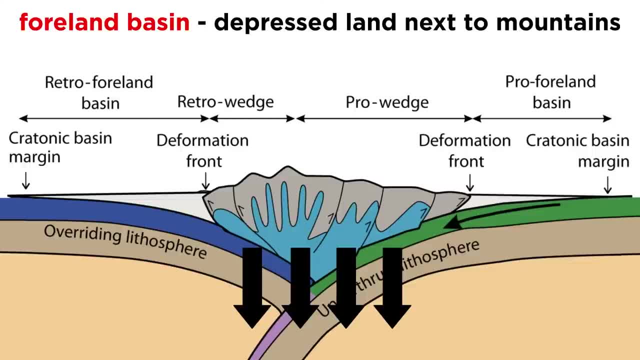 The weight of the mountain pushes the crust down into the mantle, not only beneath it but also adjacent to it, and is think of as the foundation of the ground. The Wesleyanğa này cũng t mechanisms action trên, and it is these adjacent lowlands that sink below sea level during isostatic adjustment. 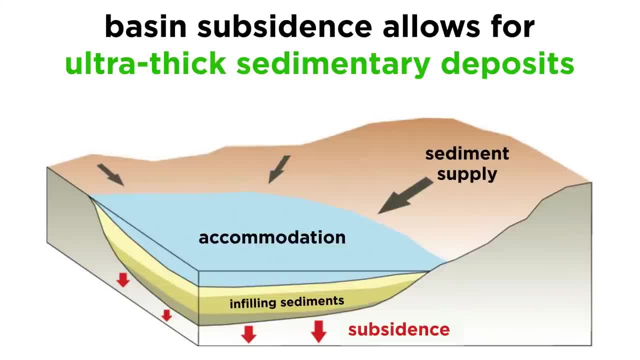 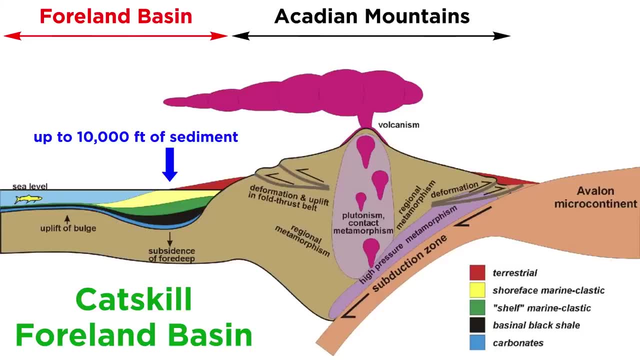 which in this case, is called subsidence Basin. subsidence is what makes the formation of ultrathick sedimentary deposits possible. For example, as much as 10,000 feet of sediment accumulated in the Catskill Foreland Basin over a period of only about 20 million years. 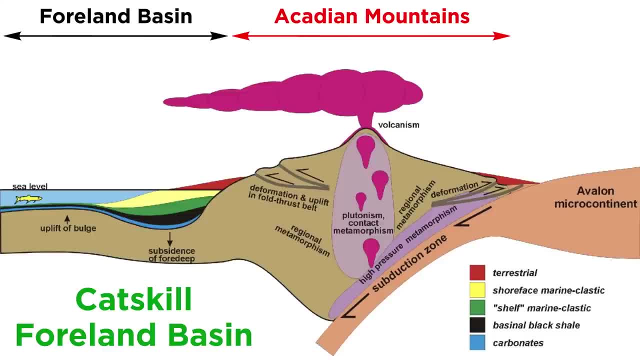 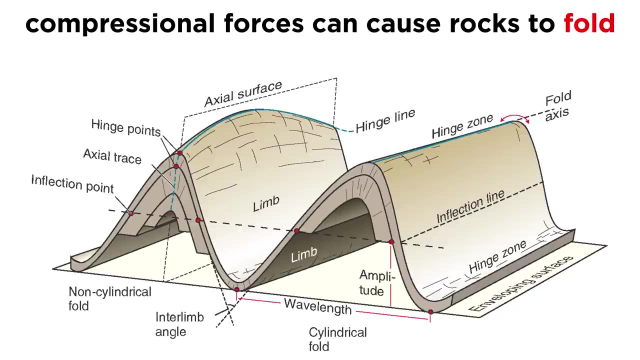 during the Upper Devonian Period. This sediment was shed from the now-eroded Acadian Mountains that existed along the eastern seaboard Subsiding foreland. basins like this have fostered deposition of some of the largest sedimentary formations in the world. In some 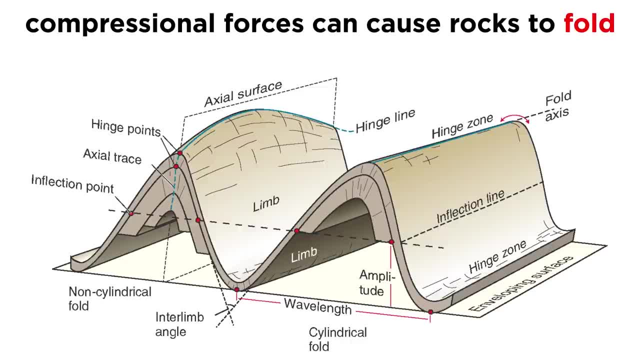 areas. compressional forces cause rocks to become folded, like a car that gets crumpled during an accident. Folding occurs when a rock is being compressed and the temperature and pressure are just high enough for the rock to be able to hold its shape. In some areas, the rock is being 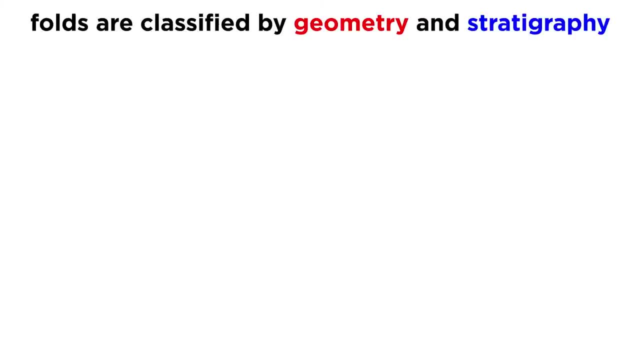 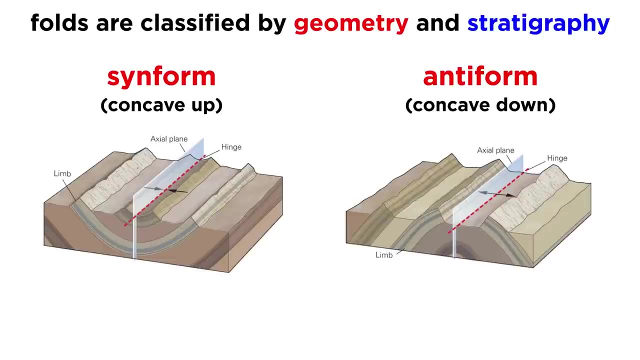 compressed and the temperature and pressure are just high enough for plastic deformation to occur. Folds are classified based on their geometry and stratigraphy, or arrangement of strata. Folds that are concave up are called synforms, and folds that are concave down are called antiforms. 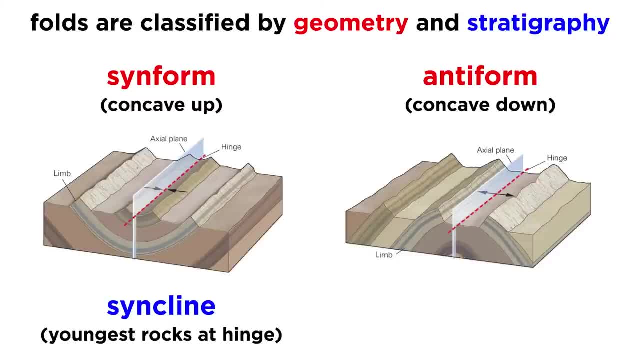 When layered rocks are folded into a synform, the youngest rocks will usually be at the hinge of the fold, which is similar to the local maximum or minimum of a parabolic function. When layered rocks are folded into a synform, the youngest rocks will usually be at the hinge of the fold. 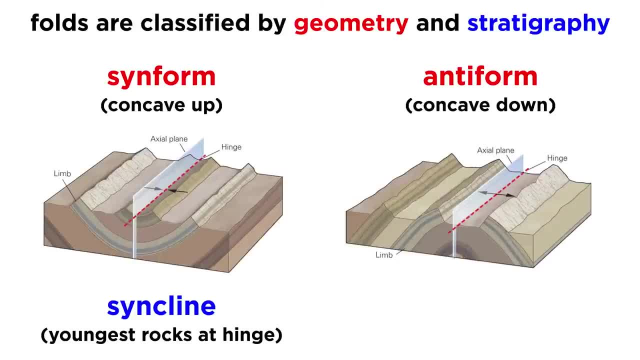 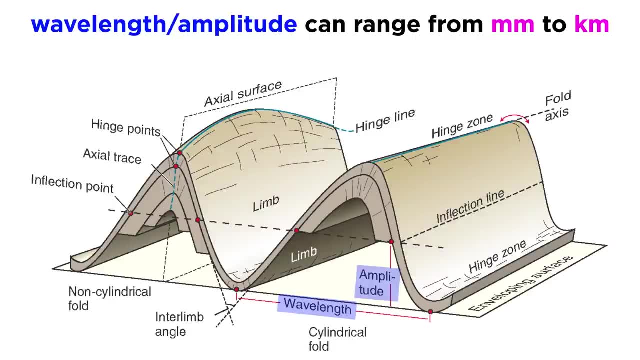 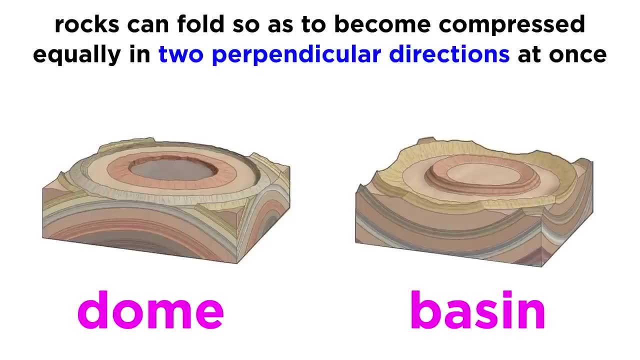 When this is the case, the fold is called a syncline. Anticlines have the oldest rocks at the hinge zone. Geologic folds can range in wavelength from millimeters to kilometers, as can the amplitude If a rock is folded in a way that compresses it equally in two perpendicular directions. 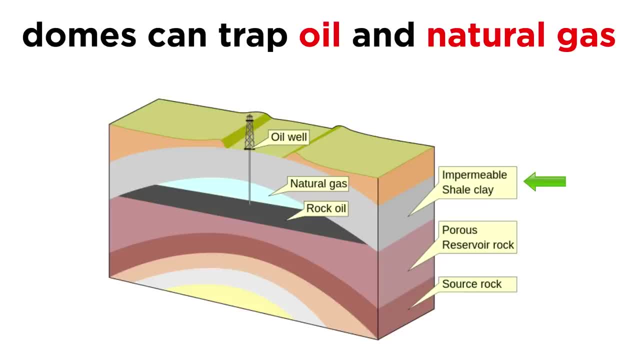 it can form domes and basins. Domes that are capped with an impermeable rock, like shale, make excellent traps for oil and gas. Hydrocarbons are positively buoyant in the earth, causing them to rise toward the surface through a rock's pore space until they are trapped by the impermeable shale dome. 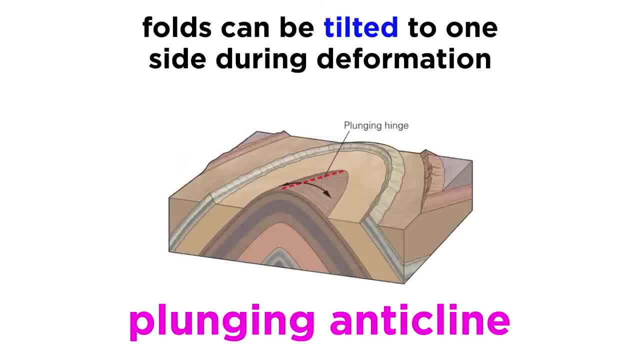 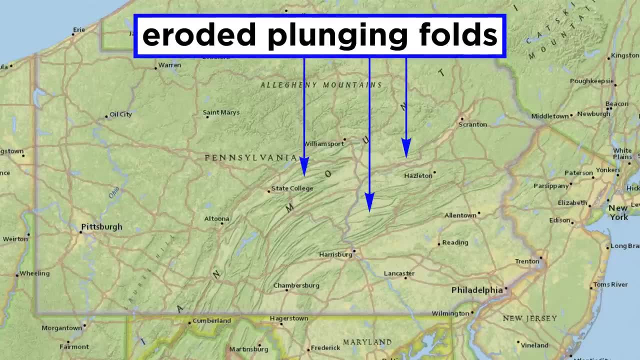 Folds can also be tilted over on their sides during deformation, becoming either plunging or inclined. The zigzag ridges of the Appalachian Mountains in Pennsylvania are also formed. The ridges in Pennsylvania perfectly represent plunging folds that have had their tops planed. 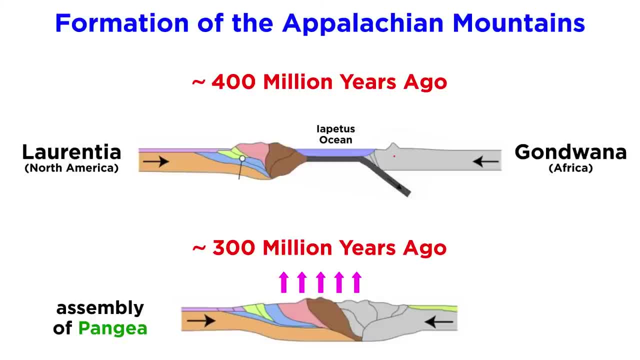 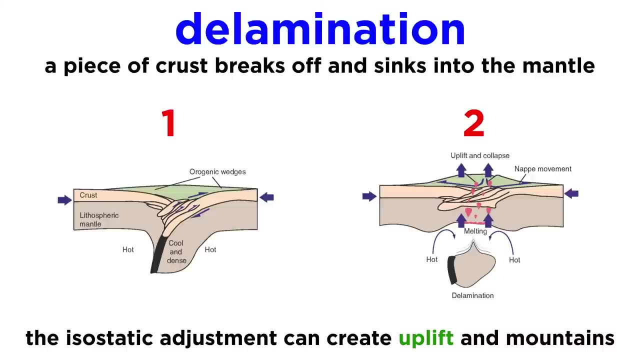 off during erosion. The Appalachian Mountains, which formed around 300 million years ago, were completely eroded into a flat plain near sea level by the beginning of the Cenozoic era. The ridges of today are caused by recent uplift due to isostatic adjustment that is hypothesized. 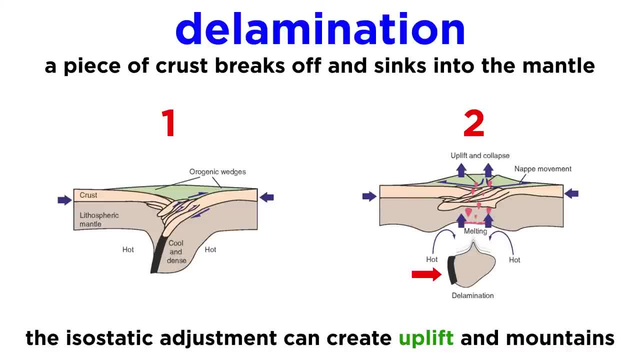 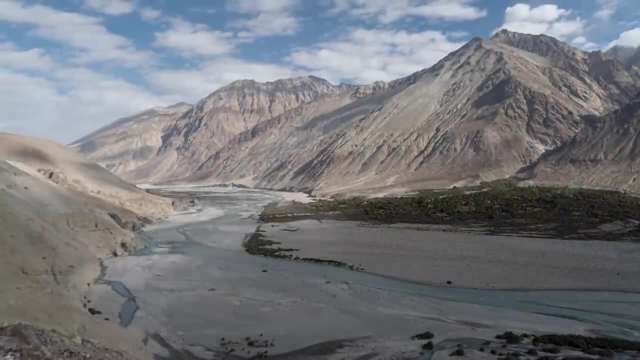 to have been caused by a piece of the bottom of the crust breaking off and sinking into the mantle In a process called delamination. Remember, whenever the crust loses mass, it bobs up. In this way they are unlike the younger Rockies and Himalayas, whose towering peaks were thrust. 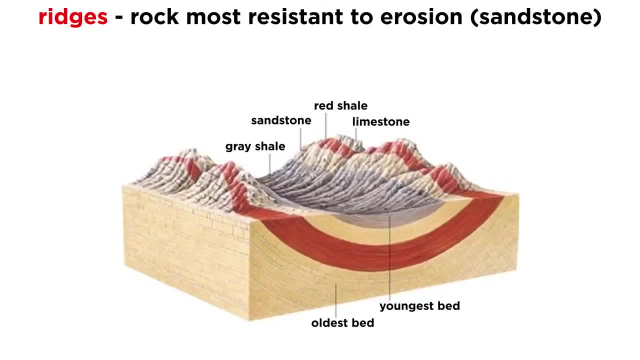 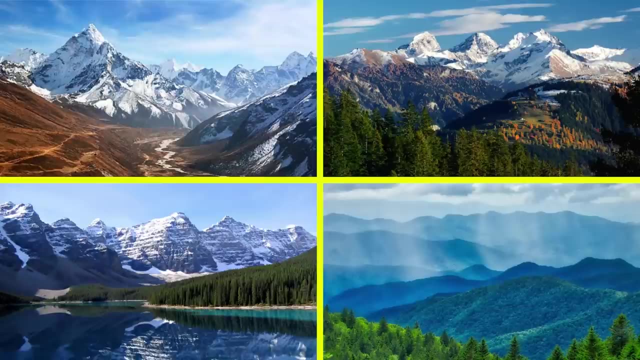 upward by the force of two colliding plates. In the modern Appalachians, the rocks that are most resistant to erosion, like sandstone, form the ridges, while the weakest and most soluble rocks, like limestone and shale, form the valleys. The most striking folded rocks are found in areas that have experienced the collision. 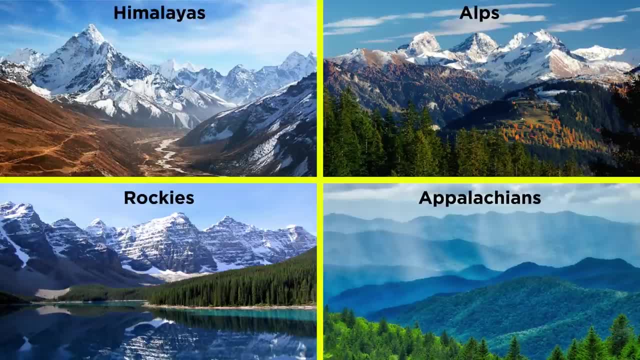 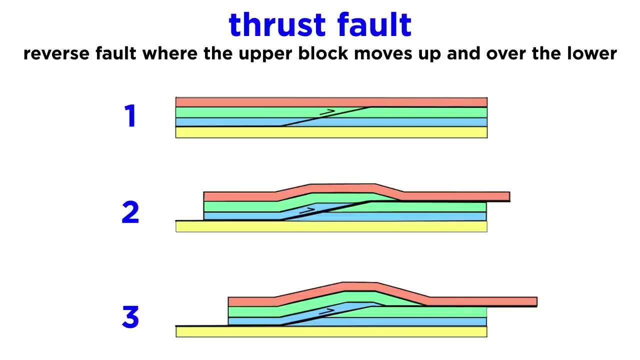 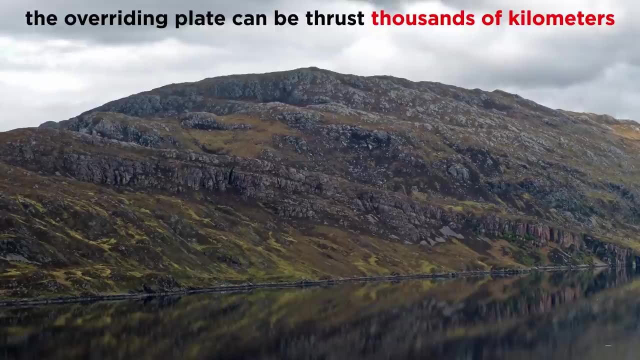 of two plates, such as the Himalayas, Alps Rockies and Appalachians. Large reverse faults, called thrust faults, are found in these locations. In some cases, the overriding plate can be thrust hundreds to thousands of kilometers over the plate it is colliding with. 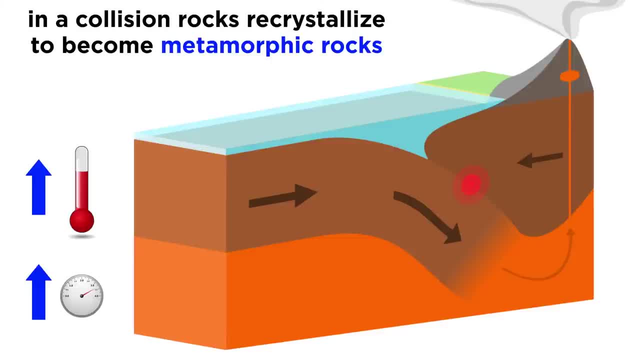 To add, it is important to know that the Cryptozoic Geological Protocol is based on the principle of the geometric element of the stratosphere. Thus, it is not the Earth. collision of two plates also cause the rocks to recrystallize and become metamorphic rocks. 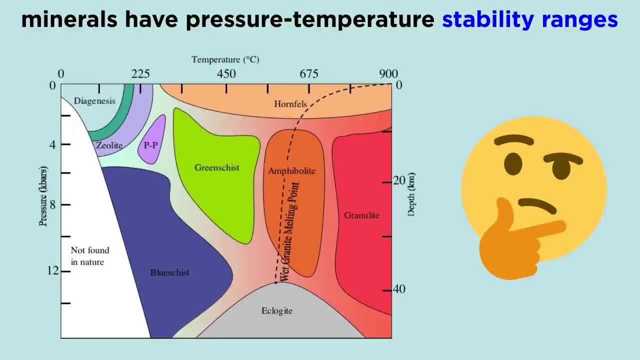 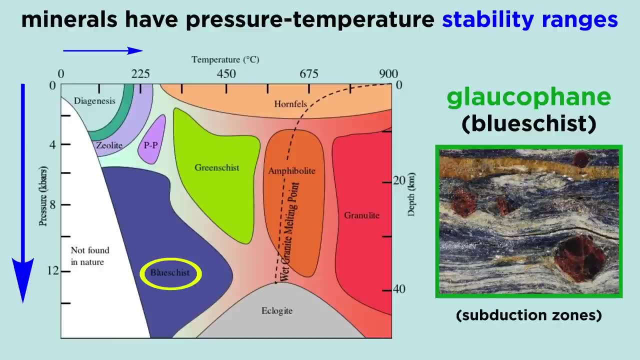 Different minerals have different pressure-temperature stability ranges and can therefore be used to estimate the pressure and temperature conditions during metamorphism. When the pressures are very high with respect to temperature, as in subduction zones, the blue mineral glaucophane forms. These rocks are called. 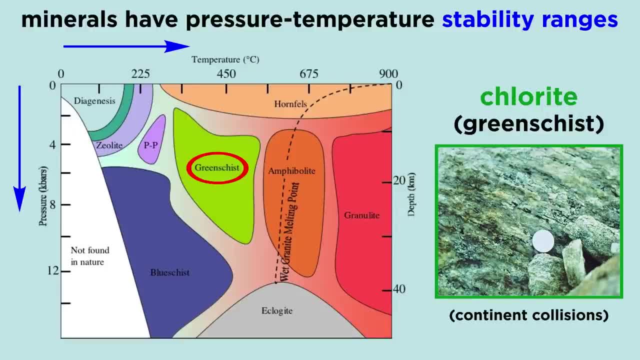 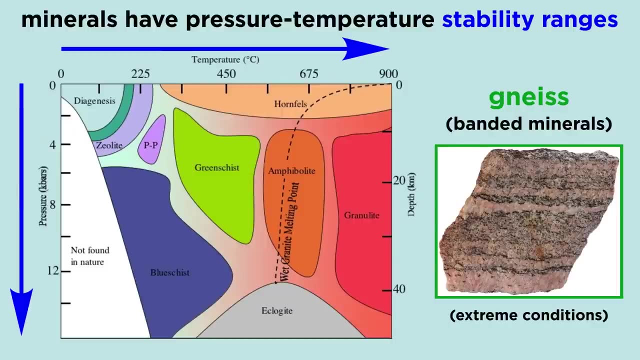 blue schist. When the pressure and temperature follow the normal geothermal gradient, as in the typical continent-continent collision, the green mineral chlorite forms. These rocks are called green schist. When both the temperature and pressure are extreme, minerals tend to become. 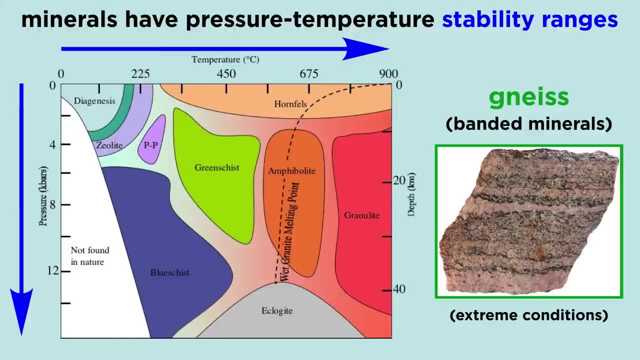 segregated during recrystallization and the light and dark minerals are banded in the rock which is called nice. Increasing the temperature much more will cause the rock to become blue schist. What is a green mineral and what is a blue schist? 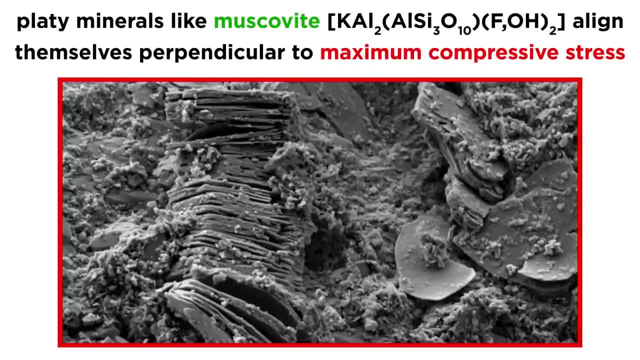 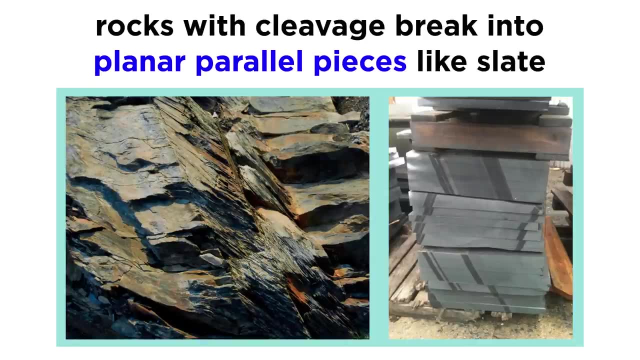 rock to begin melting In metamorphic rocks. platy minerals like muscovite tend to align themselves perpendicular to the maximum stress-creating foliation or a planar fabric within the rock that is called cleavage. When a rock has cleavage, it breaks into planar. 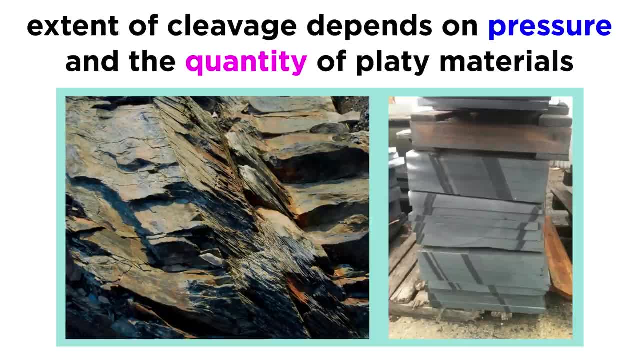 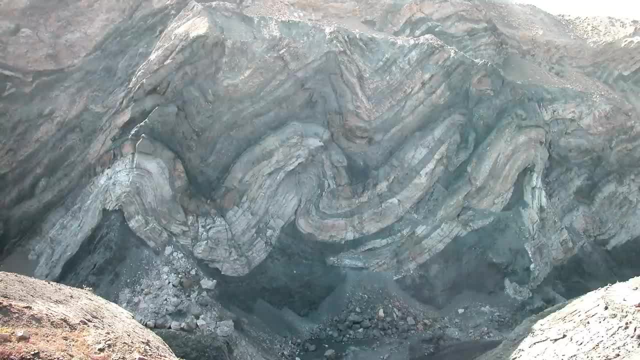 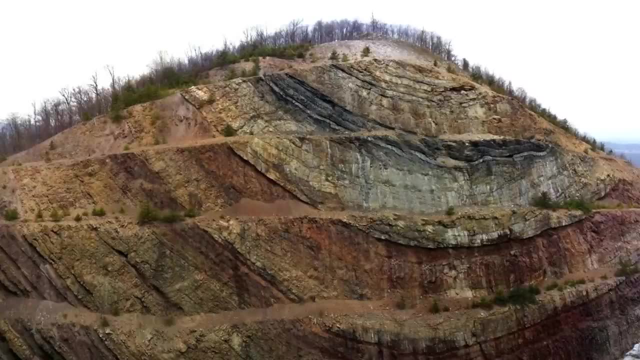 parallel pieces like slate. The extent of cleavage development depends on the intensity of the pressure and the quantity of platy materials. Features such as cleavage, folding and faulting are often present in and contribute to the formation of some of the largest and most. 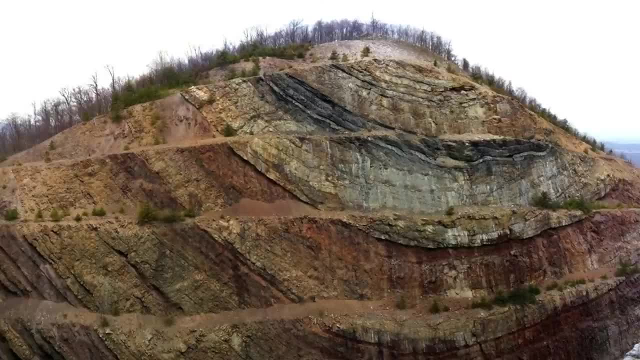 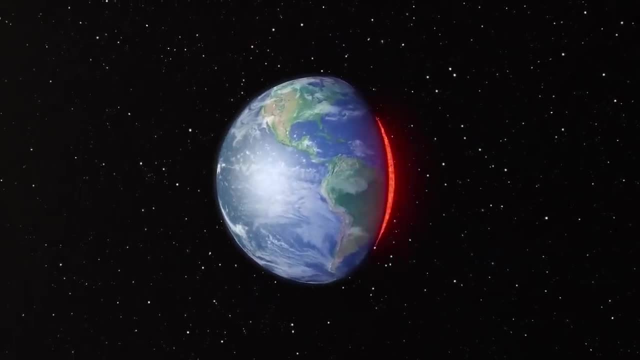 impressive geologic structures on Earth. Now that we know a little bit about how rock can react to different stresses, we are ready to learn about the structure of the Earth in considerable detail, from the surface all the way down to the core. so let's move forward and